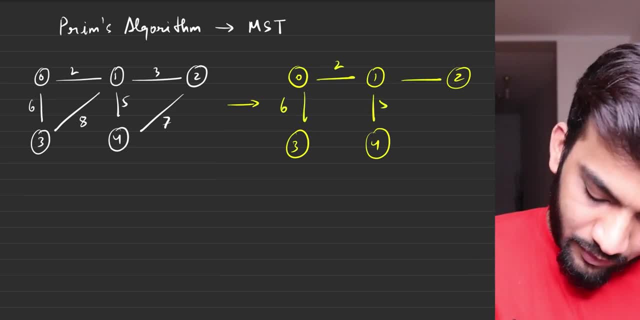 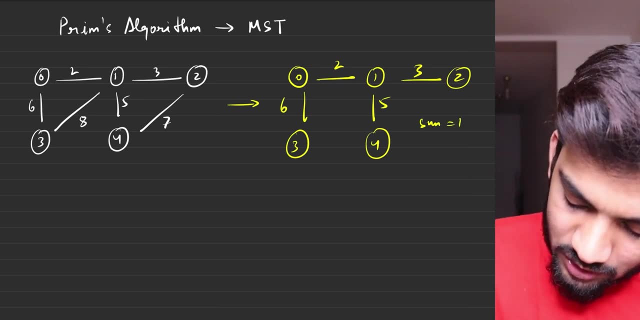 and if you connect these guys, it'll be 6, 2,, 5, 3.. And if you sum them up, you'll get 6 plus 2, 8 plus 3, 11.. 11 plus 5, 16.. So 16 is what the summation is. So Prim's algorithm does help you to find. 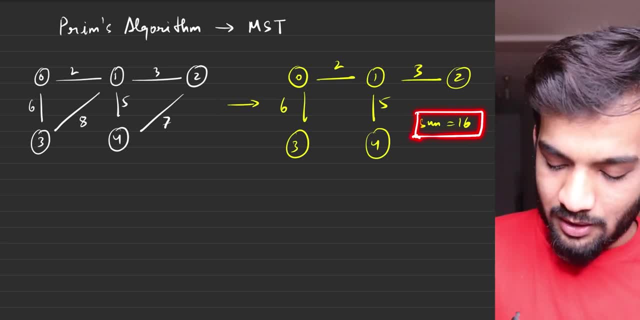 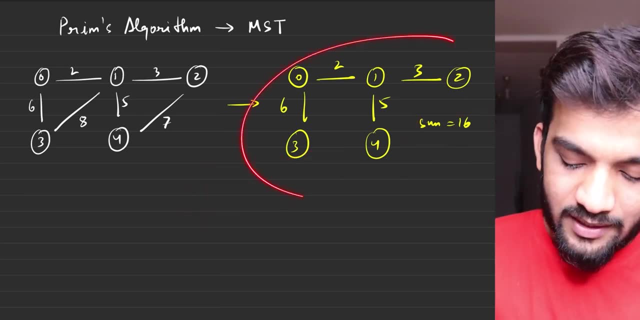 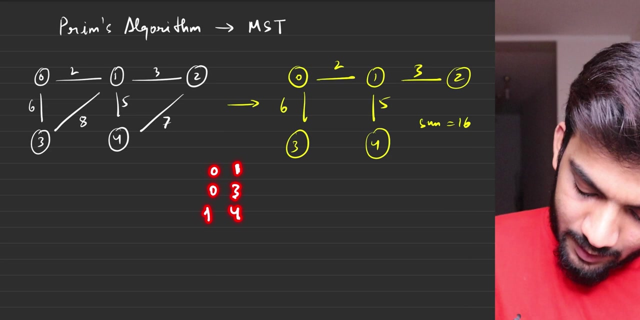 this particular summation, which is nothing but the MST's weight. We can usually call this as MST's weight or even, if you want, the edges, like for an example: the edges involved in the tree are 0, 1,, 0, 3,, 1, 4, and 1, 2.. These are the n minus 1, or 4,. 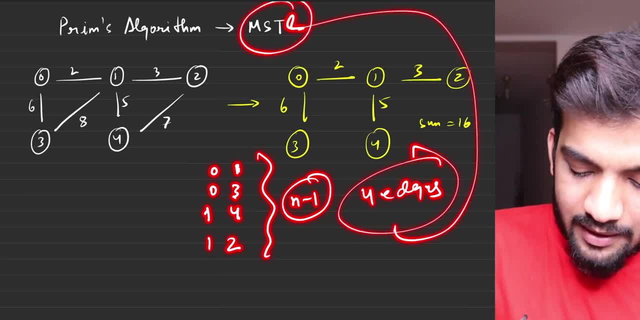 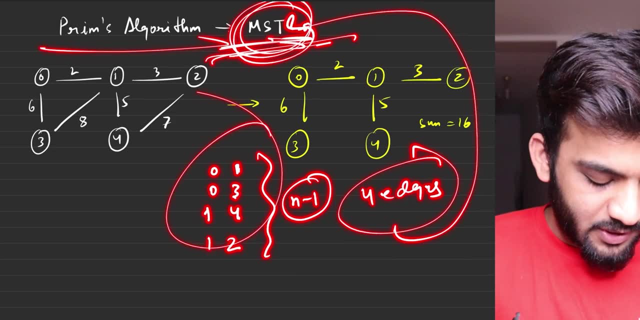 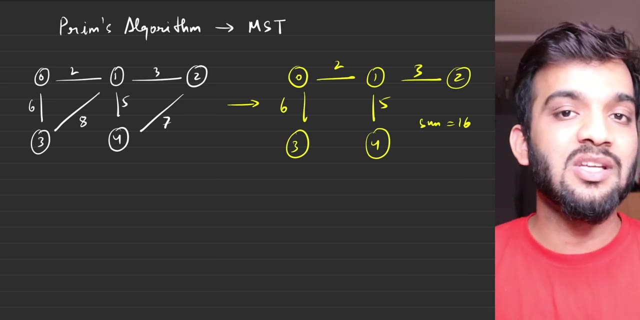 which are the edges, which are involved in MST, So you can also get this particular thing if you are looking for. So Prim's algorithm does help you to find the sum as well as the particular tree which is indeed the MST. So, in order to understand Prim's algorithm, we will be using this particular 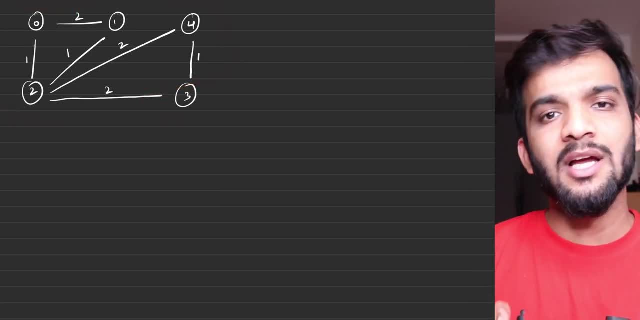 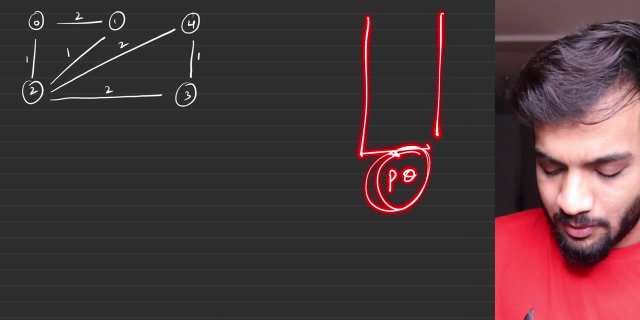 graph. So, before starting Prim's algorithm, we will be requiring a couple of initial things. One is a priority queue- is what I'll require, I'll tell you while I explain the algorithm. And the other one is a visited array, which I'll be. 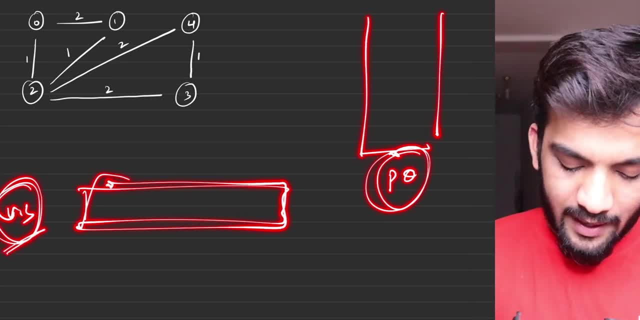 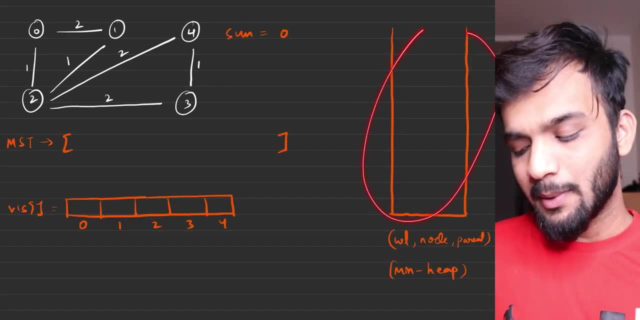 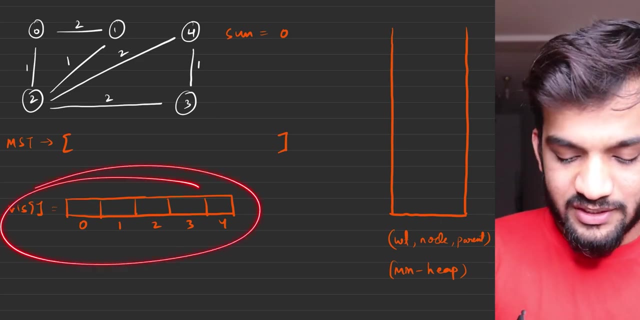 requiring again. I'll be telling you why will I be requiring a visited array while I explain this particular algorithm. So the initial configuration will have a priority queue or a minimum heap in which I'll be storing the weight, the node and the parent. Along with that, I'll have a visited. 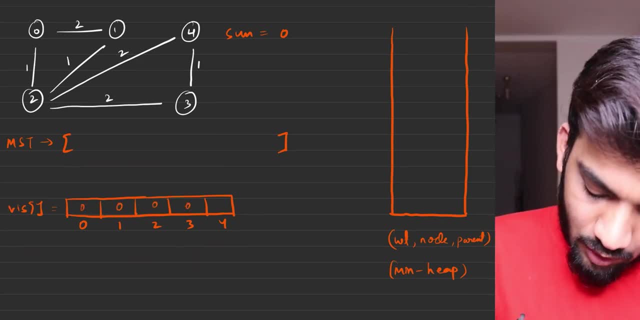 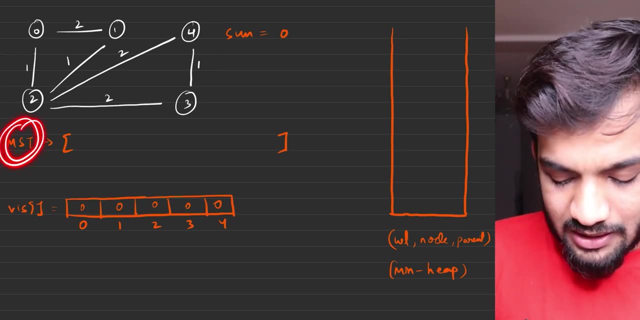 array which will be initially marked with unvisited, with all the nodes, And we will have a sum of 0, which will count the MST's edge weight And I'll have an MST list which will be storing all the edge which are: 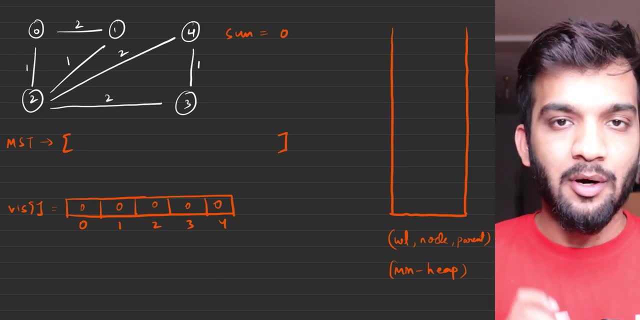 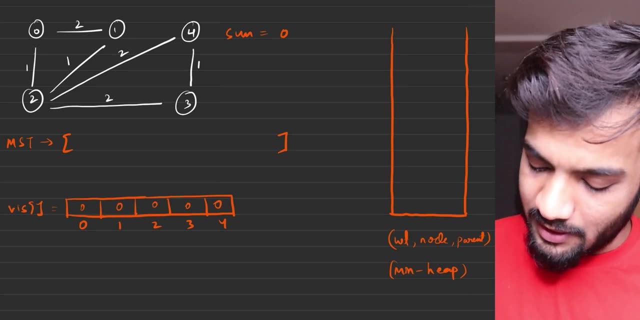 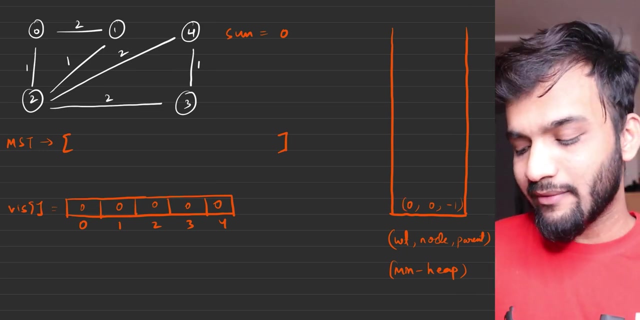 part of the MST. So initially, remember, you will start off with any given node. It can be any given node, that is your choice. So what I'll do is I'll start off with something like 0 with the weight, 0 with the node, and I can say: the parent is minus 1.. Remember this, This is what I will initially. 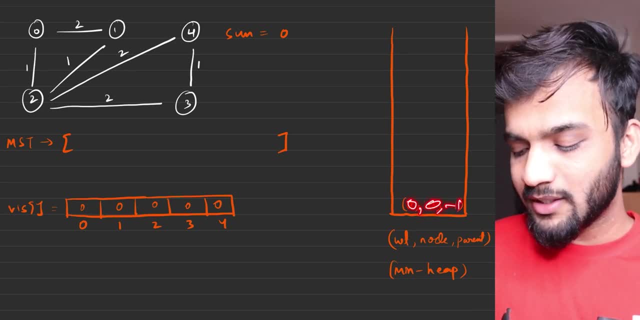 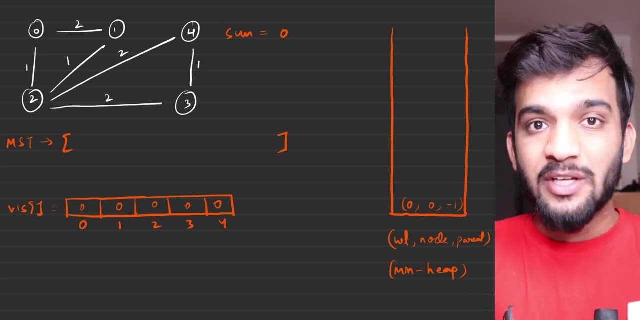 insert 0, weight 0. node minus 1 as the parent. Okay, now we will start the iteration. Remember: no visited mark. We just put it into the priority queue. That is the initial configuration. Now we start the iteration. So while we start the 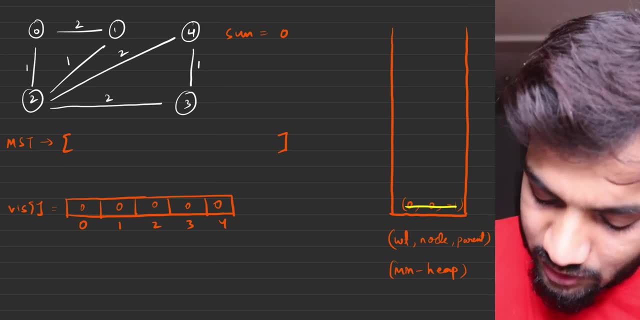 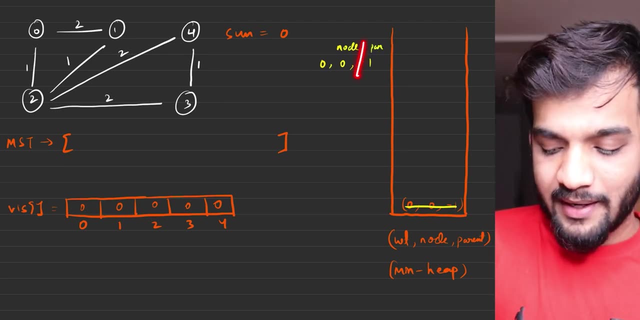 iteration, we get only element on the priority queue, which is at the top, which is 0, 0, minus 1.. So this is the node, This is the parent. So whenever the parent is minus 1, it means it's not. 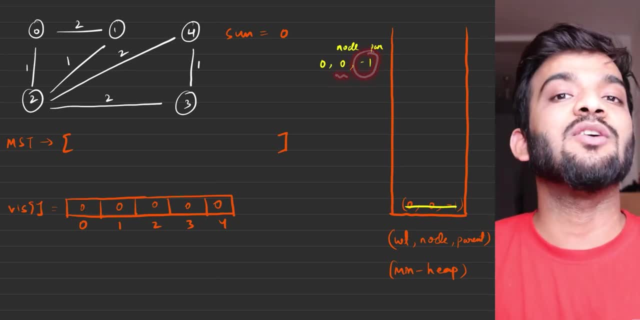 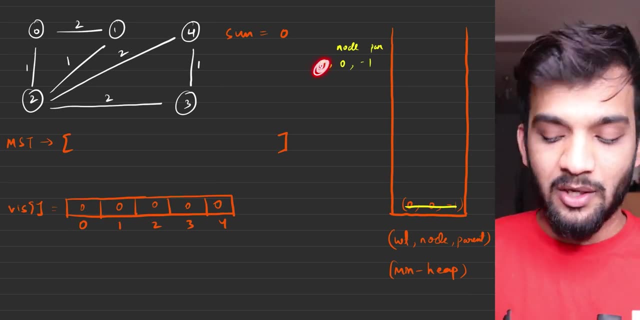 an edge. It's the first node. Parent minus 1 means it's the first node, So do not add it into the MST. Do not add it into the MST. Also, there is no edge weight because this is the first node. That's why. 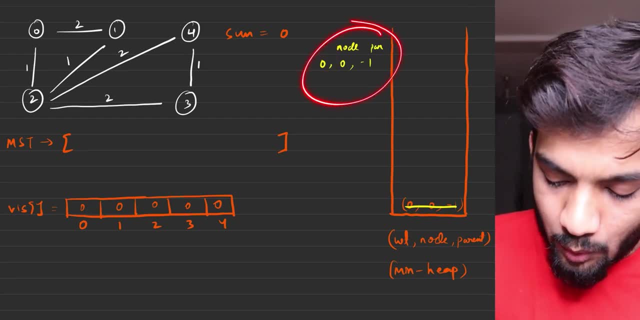 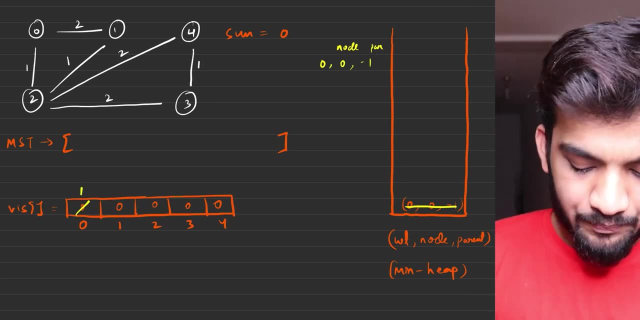 there is no edge weight as well, So we have the first node as 0.. Make sure you go across and mark it as visited. Mark it as visited Now. stand at 0 and look at the adjacent nodes. So when you stand, 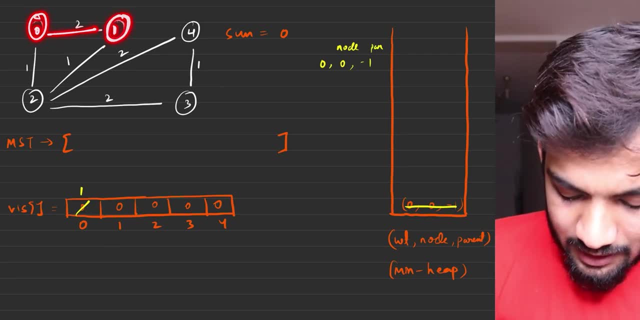 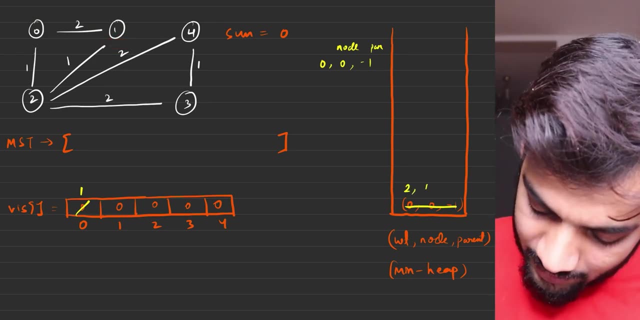 at 0,. you look at one of the adjacent node as 1, and that's still unvisited. So what you do is you take the edge weight as 2.. So 2, 1 comes from 0. So basically, you are standing at 0. So you took. 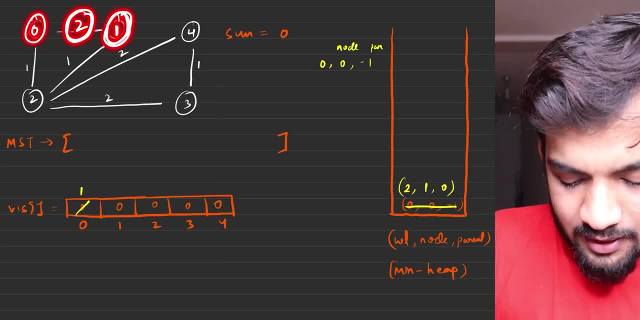 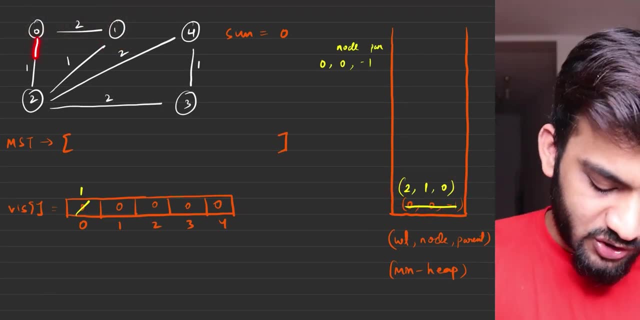 the edge, weight 2.. You took the node 1, and it came from 0. So, basically, this is the edge that you took, Perfect Done Next. this is also connected to 0. So what you will do is you will. 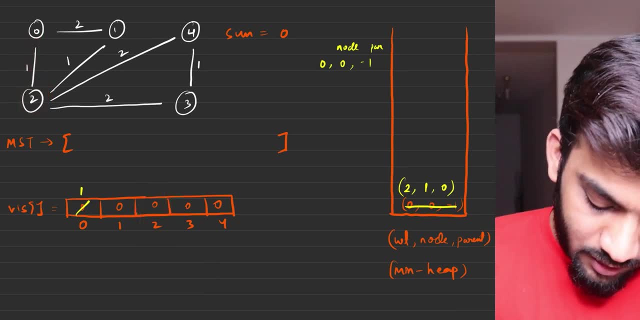 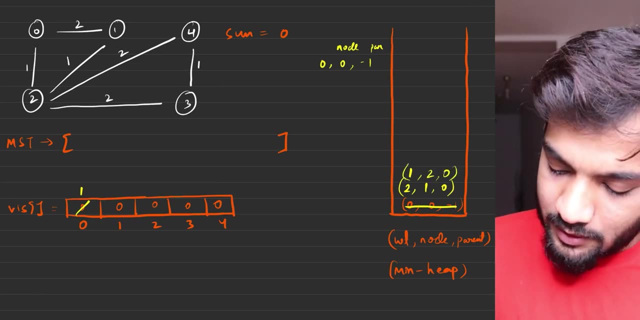 see, is this unvisited? Yes, So simply take 1 as the edge weight. So I'll take 1 as the edge weight. Came from 0. So what I did was I take both the guys who are directly connected to 0. But please. 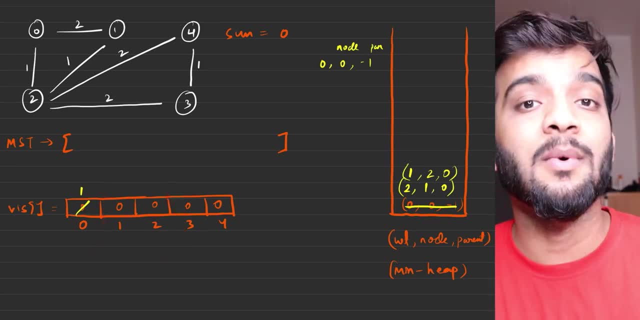 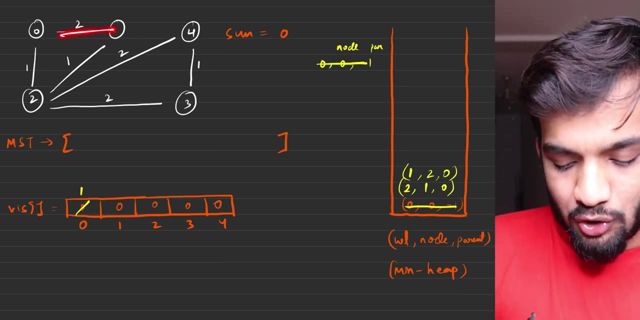 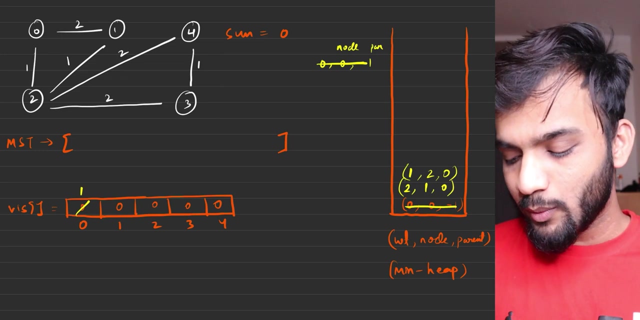 do not mark them as visited. Please do not mark them as visited. Okay, So I've taken it, So I can say the first iteration has been complete and I have pushed on all the adjacent nodes into the minimum heap data structure. Now, what does minimum heap data structure say? We will always. 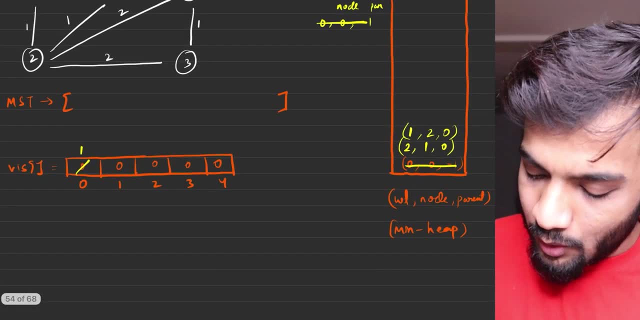 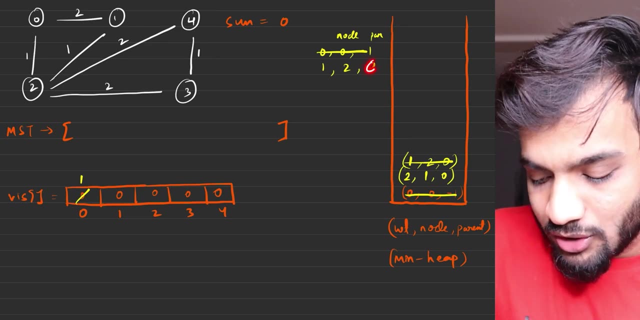 have the least weight at the top. So I'll get the least weight, guy, which is 1 comma 2 comma 0, so 1 comma 2 comma 0.. This time you're getting an edge 0, 2.. You're getting an edge 0, 2.. So it. 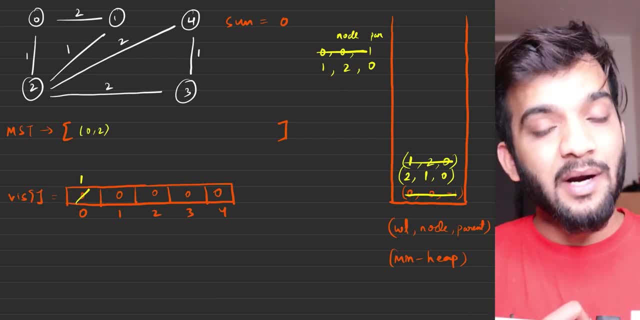 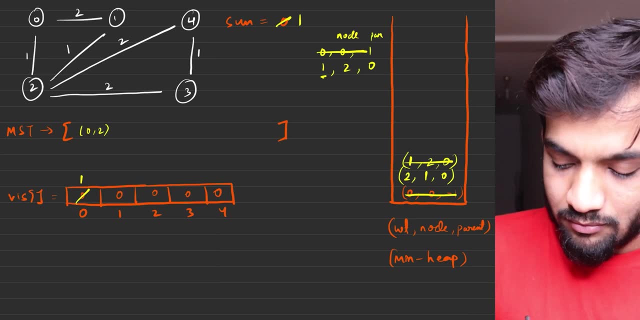 will be a part of your MST. 0,, 2 is a part of your MST And whatever is the edge weight, you'll go and add it on the sum Done. Now you have the node as 2.. So go to the 2 and say you are visited. 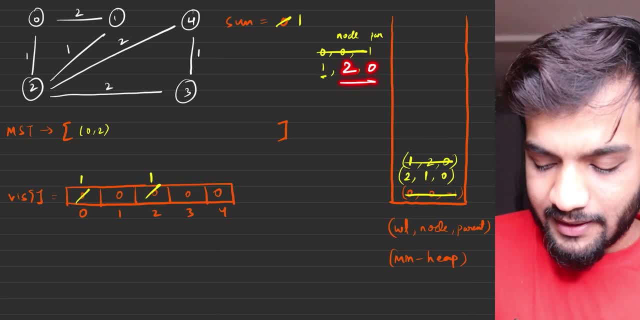 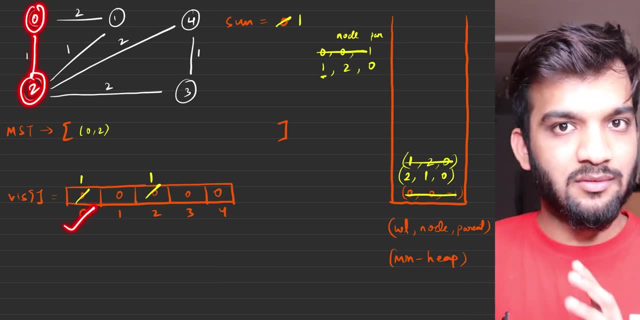 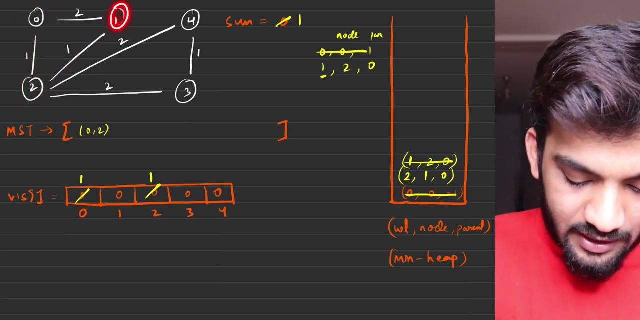 Right Next. So you have taken 0,, 2, and that is what you have taken. Now stand at 2.. So you stand at 2, and you look at 0. But 0 is already visited, So do not look at 0.. You look at 1.. 1 is unvisited. Yes, 1 is unvisited. If you stand at 2, 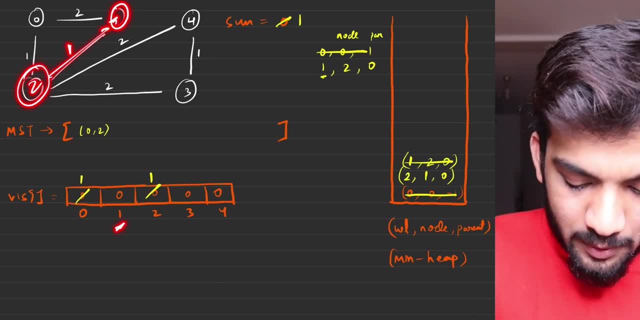 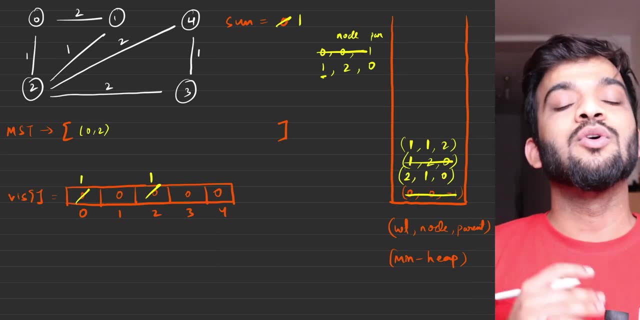 and look at 1, it's still unvisited, So it's an edge weight of 1.. So you can again take 1,, 1, and this time you came from 2.. And this time you came from 2.. So you can easily take it off, Okay. 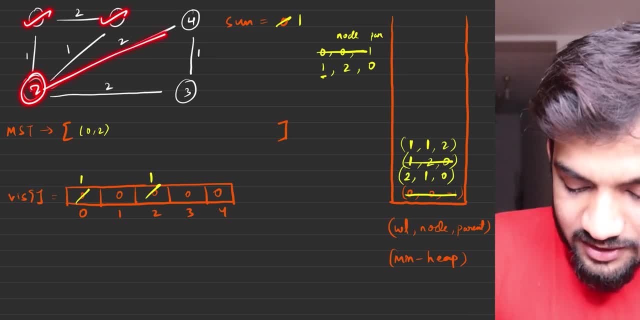 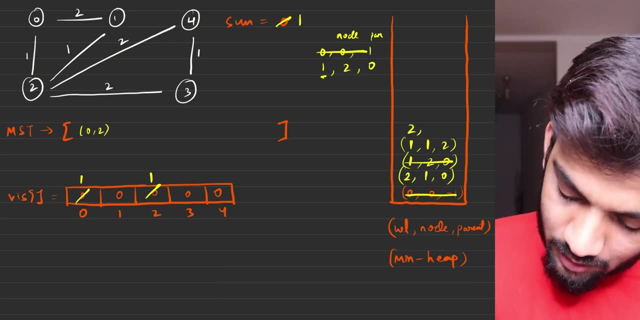 Next, If you're standing at 2,, 0 is done, 1 is done. Next adjacent is 4.. It's unvisited So you can again take it. So 2, 2 is the edge weight, 4 is. 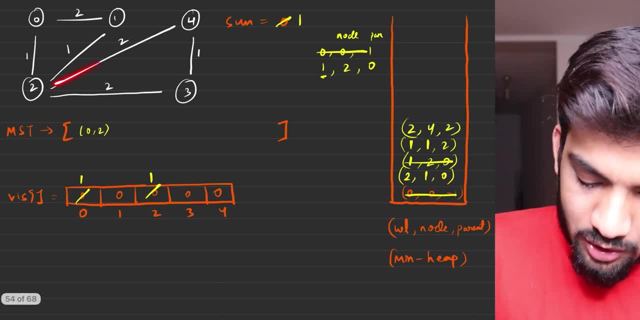 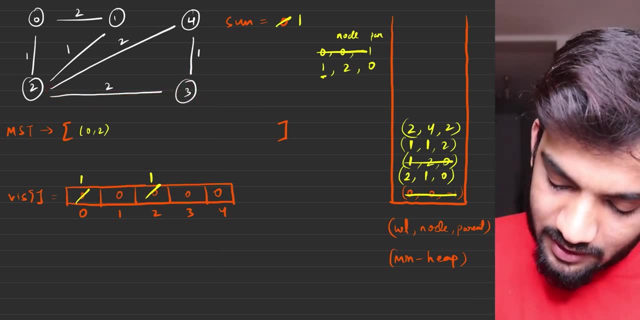 the node And you're coming from 2.. So this is what you'll put it into the priority queue. Do I have anyone else? We have a 3.. Yes, we have a 3.. So what I'll do is I will this time take the edge weight. 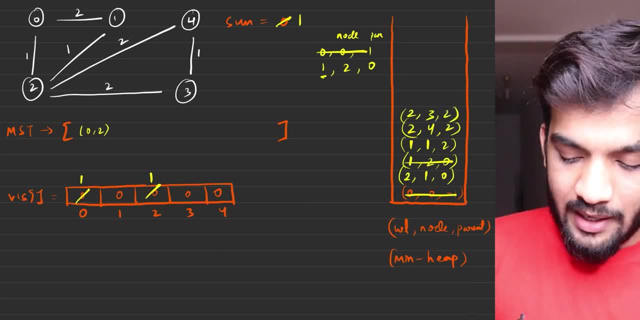 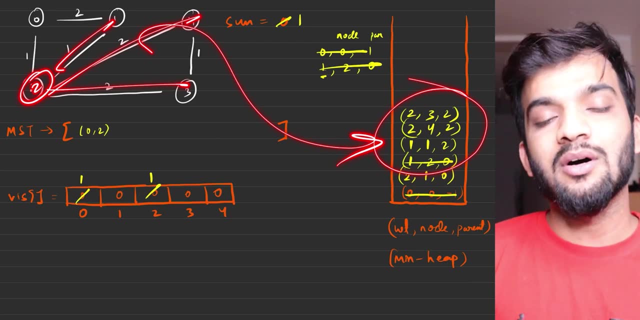 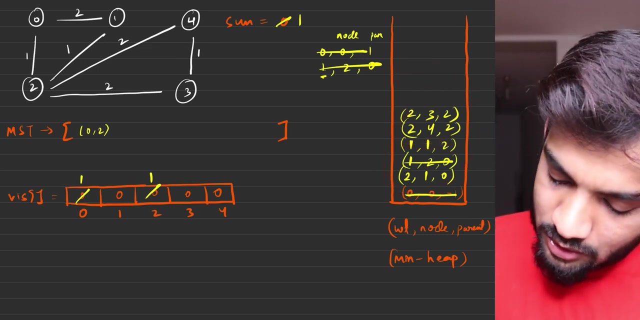 2.. We will take. 3 came from 2.. Perfect, So apparently this is also done, And I made sure that the edge weight is equal to the priority queue. Next, Take the next smaller guy, Out of which, which is the next smaller guy? Obviously 1, 1, 2.. So take 1, 1, 2.. So 1, node 1, parent 2.. 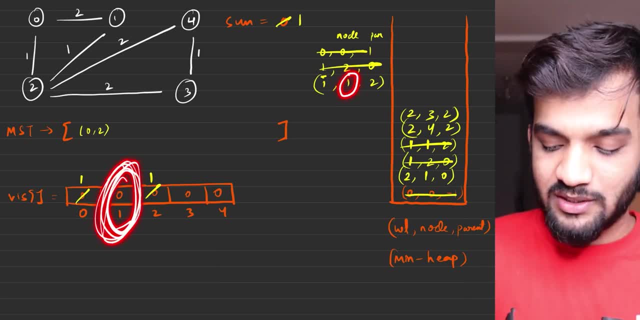 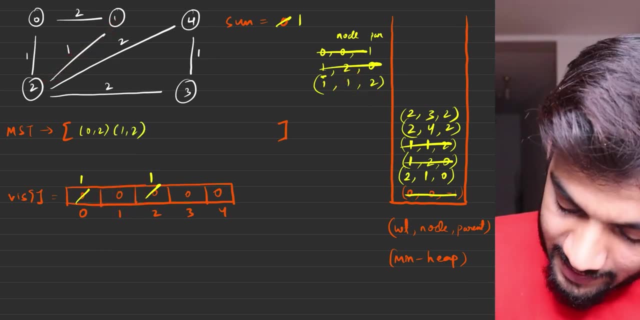 Go and look at the node 1.. Is it unvisited? It is unvisited, which is 1, 2, which is nothing but this edge. So I can say I'll take this edge now. 1, 2 is the edge, Or rather 2, 1.. You can call it. whatever, Because 1, 2 or 2, 1.. Both are same, So I'll take this edge now. 1, 2 is the edge, Or rather 2, 1.. You can call it whatever, Because 1, 2 or 2, 1.. Both are same. 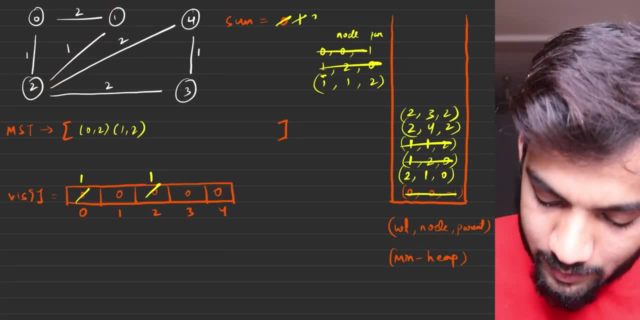 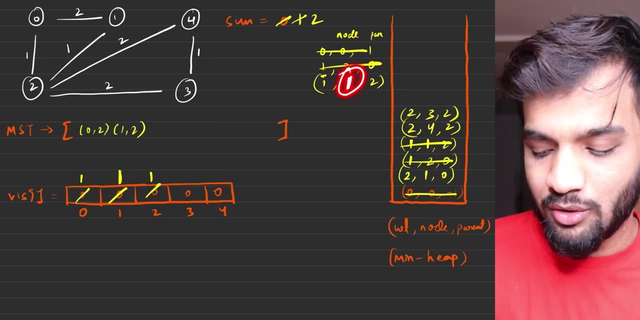 Right, And the edge weight is 2.. Sorry, edge weight is 1.. So you add 1 to it, You'll get it as 2. And at the same time make sure you mark it as visited. So apparently now 1 is also visited. 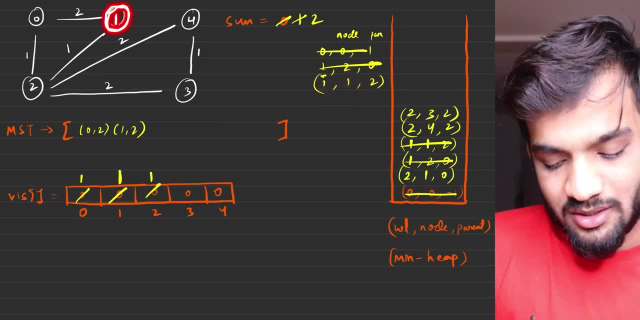 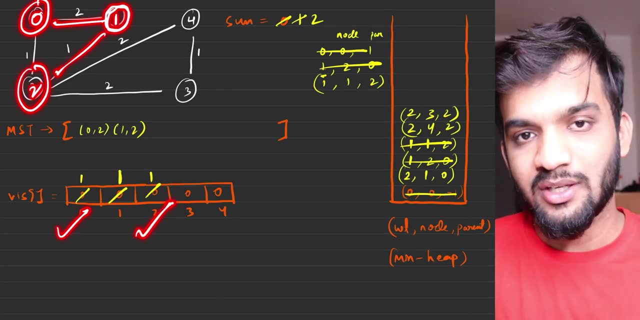 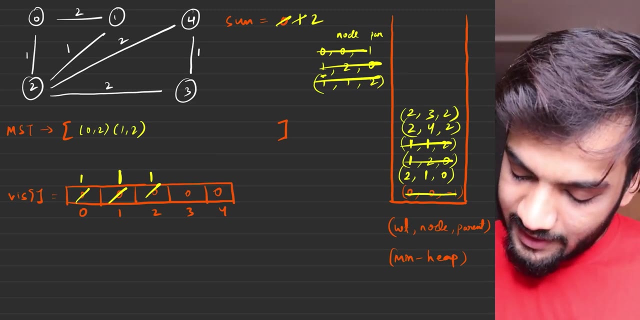 Now stand at 1 and look at its adjacent. Its adjacent is 0,, which is visited. Its adjacent is 2,, which is visited. So there are no other adjacent. So thereby I can say the iteration has been completed. Now let's look at the next one. What is the next one? 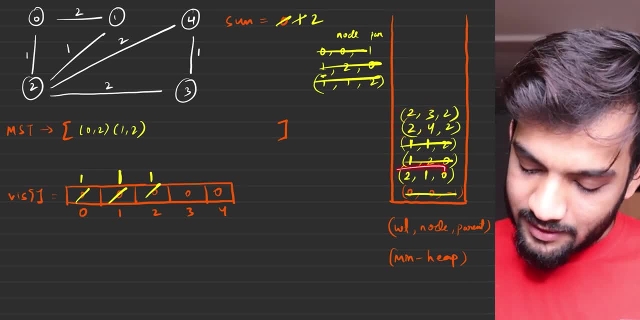 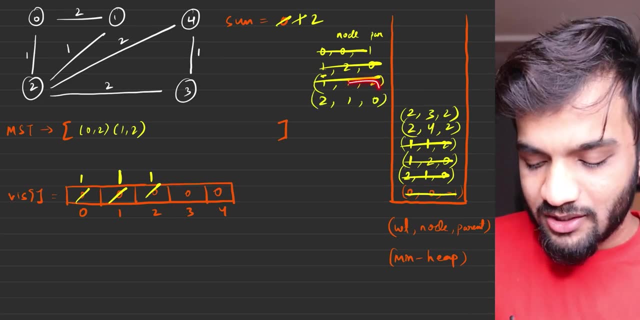 Which I'll get. All of them are same Separately, we will get this guy. So 2, 1, 0.. 2, 1, 0.. But before moving ahead and adding this to your sum or to the MST, we see, hey, wait, The node 1.. 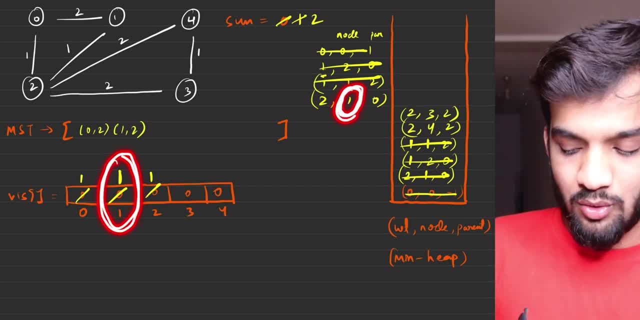 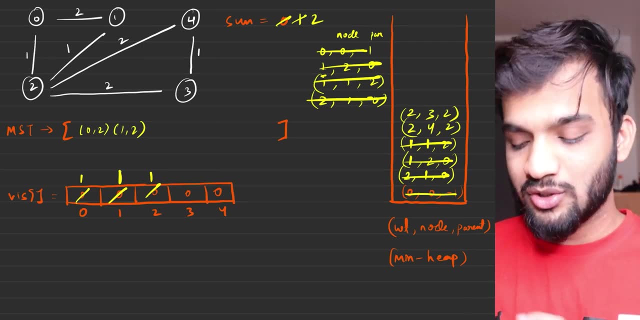 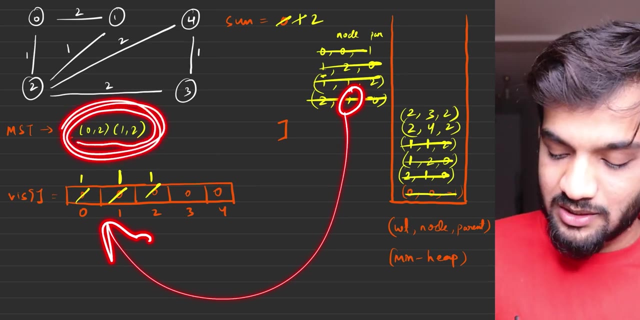 The node 1 is already visited, So you do not add it. Yes, You do not add it And you do not do any adjacent operations. If the 1 has all the adjacent operations, you do not do any adjacent operations. already been visited, which means it's a part of your mst. it's a part of your mst, so do not add it. 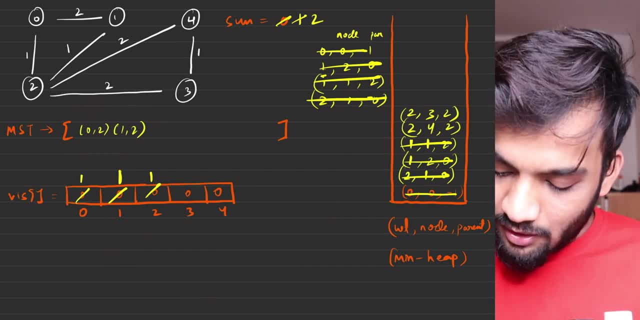 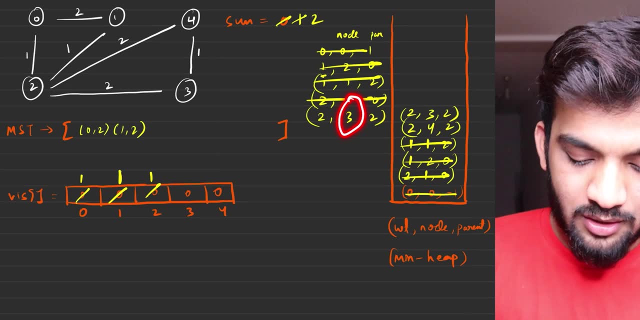 right next you find out the next guy. so out of these two guys we'll take 2 comma 3 comma 2. so 2 comma 3 comma 2 this time, which is the node 3. so go and mark 3 as visited next. this is the. 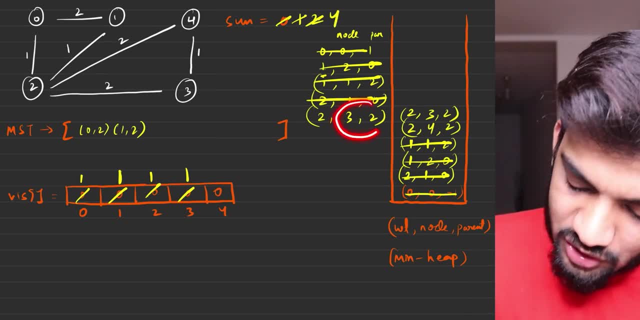 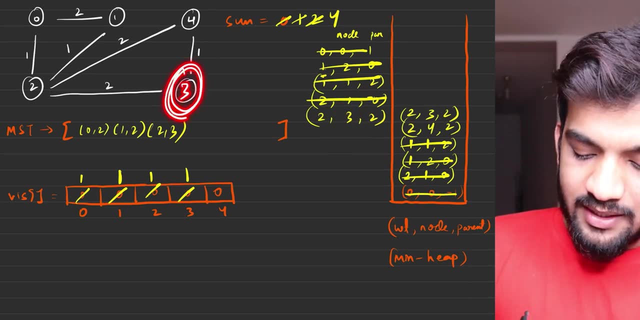 edge weight. go and add it, so this will be 4. next, this is the edge 2, comma 3. go and add it to your mst. now you're standing at 3. stand at 3. look at its adjacent. one of the adjacent is 4 with 1. 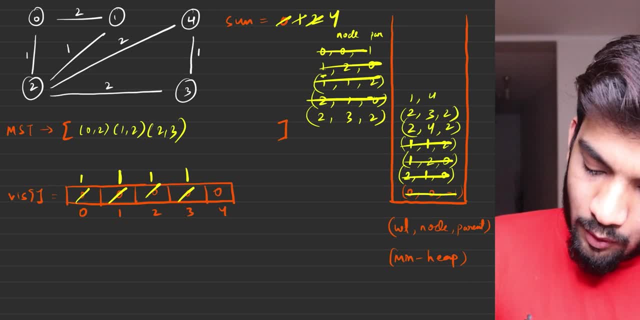 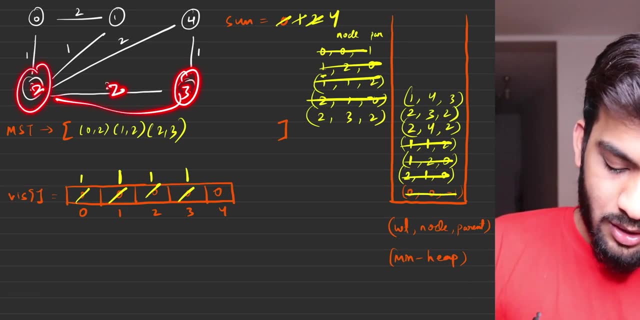 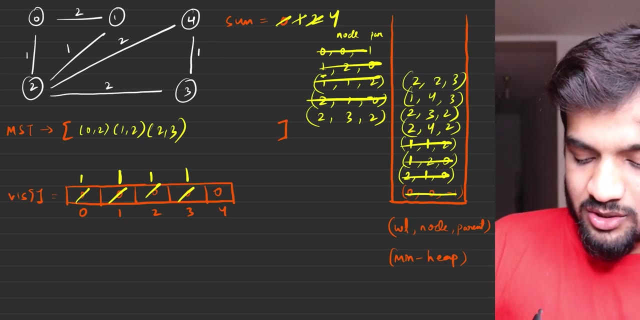 so really you can add it. 1 comma 4 comma 3. i've added it. and for 3, the other adjacent is 2, so 2 comma 2 comma 2. uh, 2 comma 2 came from 3. you've added that into the priority queue because. 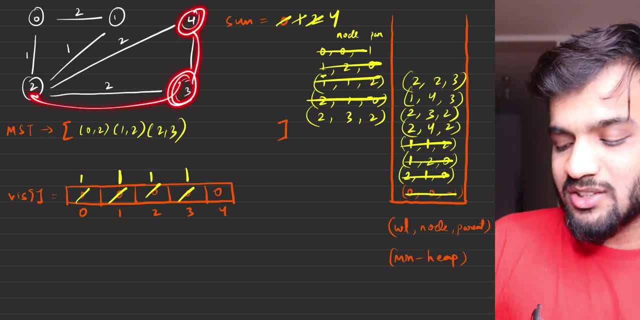 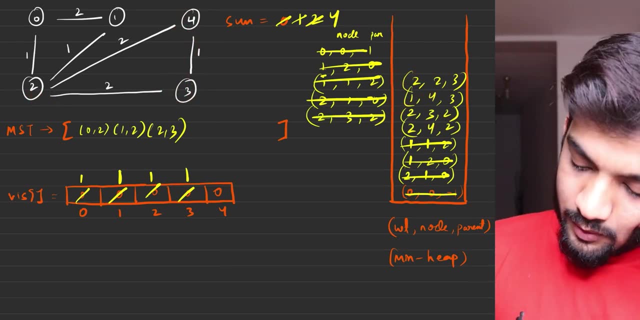 for this guy. this was one of the adjacent and this was one of the adjacent, so i've added both of them. i can say my iteration has been completed. now, quickly, which one is the smaller: one comma four, comma three. so take it out: one comma four, comma three is for unvisited. yes, go. 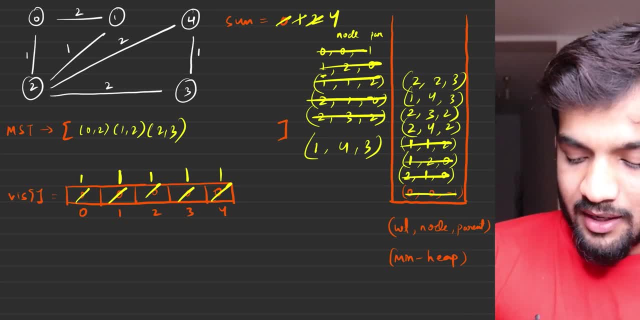 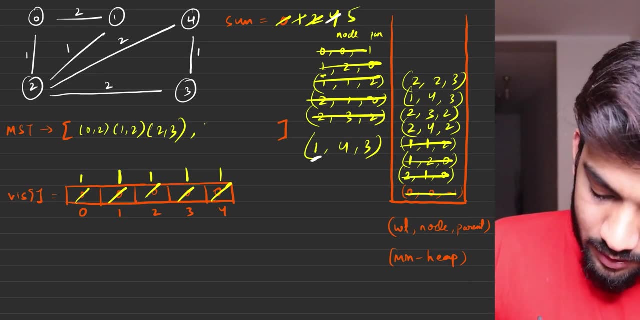 across and mark it as visited. once you've marked it as visited, what you'll do is you'll take this one, add it into this and this will become five, and the three comma four is the edge which will be added to your mst. now what you'll do is you will go ahead and say: okay, i, i was at four, so. 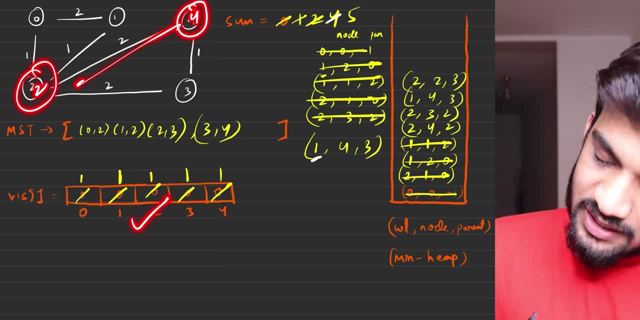 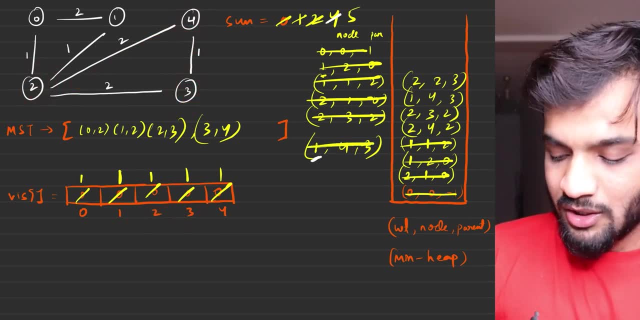 i'll stand at four and i'll look at two, but i see two is already visited. i'll not do it. i'll look at three, which is already visited. i'll not do it. so apparently i'll not get any other adjacent nodes, so i can say: one comma four, comma three is done, which is the next one i'll get. i'll get two comma. 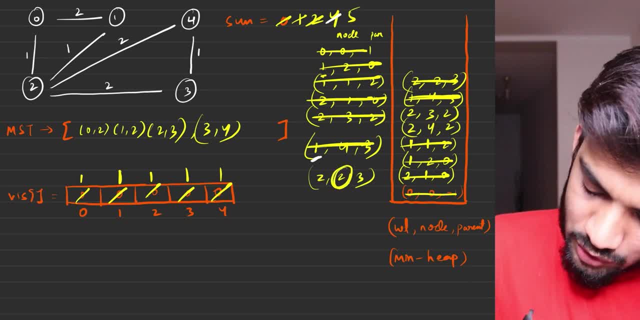 two comma three. and when i get two comma two, comma three, i see two is already visited, so i'll also not do anything. so two comma two, comma three is done. next i'll get two comma three, comma two, and i'll see three is also visited. so nothing to be done. 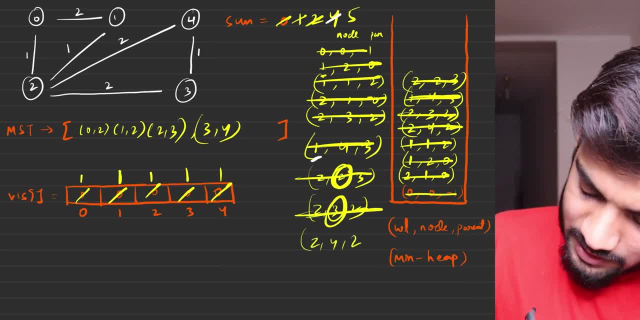 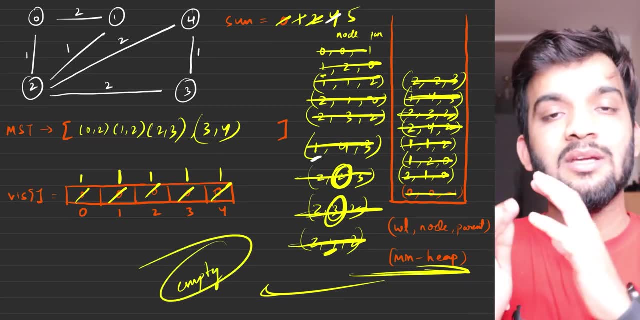 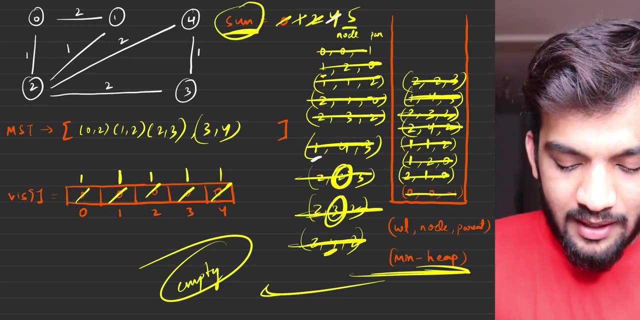 next i'll get two comma four comma two, two comma four comma two, and i'll see four is also visited, so nothing to be done. ultimately your mean heap is empty. and once your mean heap is empty you can say that it's over. rim's algorithm is over and the algorithm has got the mst sum as five, and this is 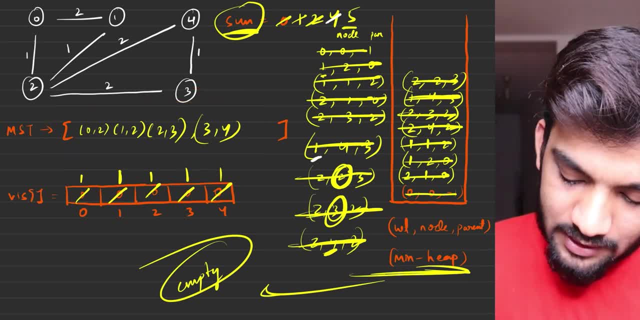 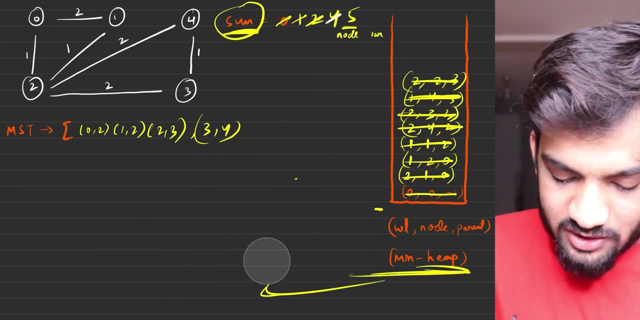 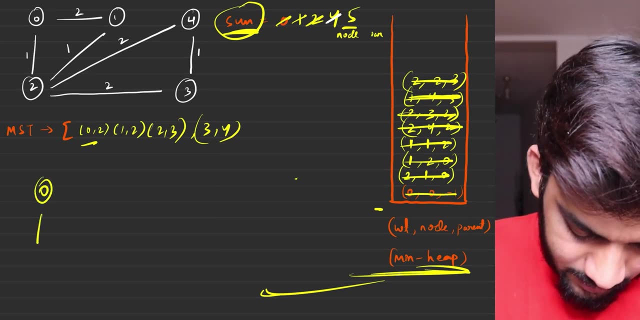 where the mst is stored. so now what i'll do is i'll quickly erase this off and try to draw the mst so that the idea is clear to you. let's see if the mst was formed properly or not. so which is the first edge, zero to two. so let's take zero and then take two, which is an edge weight of one. next, 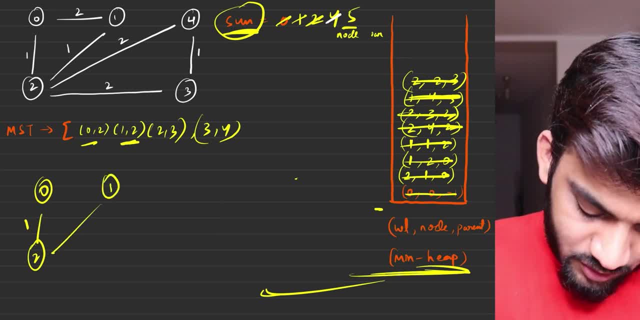 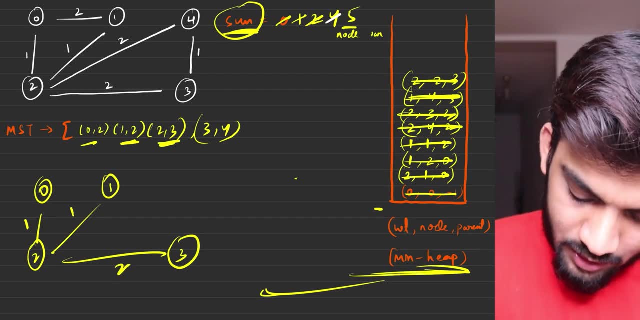 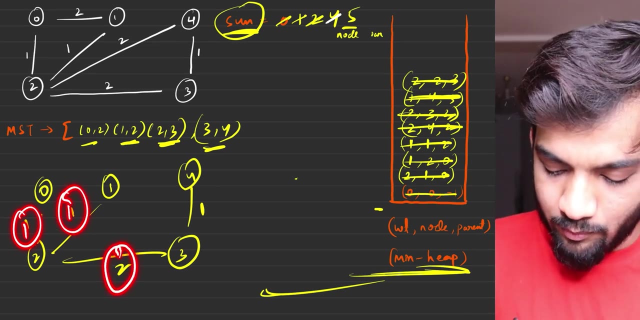 is one to two, so next is one to two, with an edge weight of one. right next is two to three. so which is this? with an edge weight of two. next is three to four, with an edge weight of one. so it's like one, one, two plus two, four plus one, five, which is your sum and which is your mst as well. so what i have? 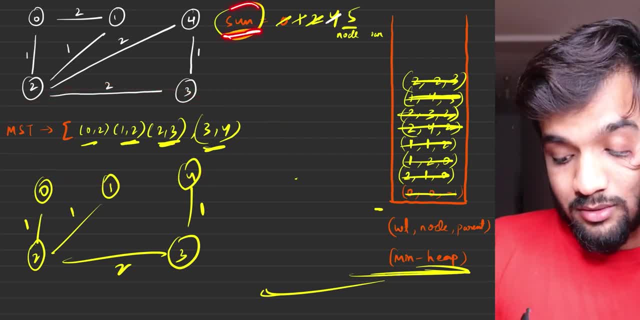 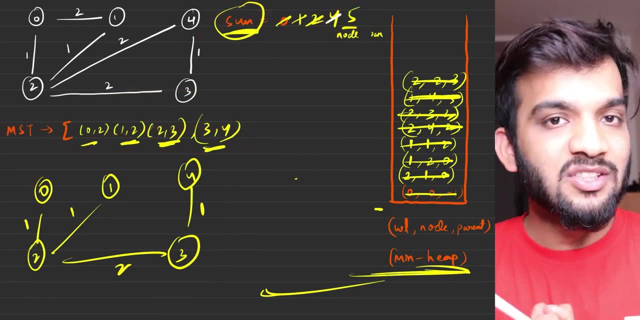 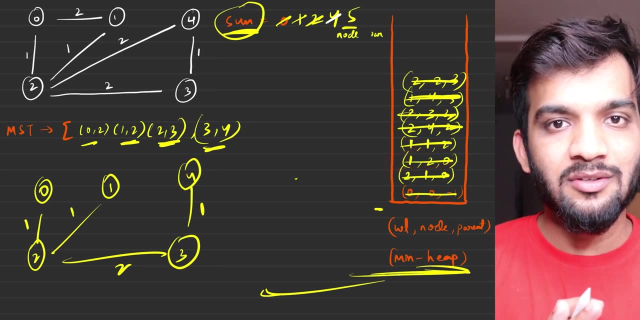 done is. i have successfully found the sum of the mst. also, i found the mst which is stored over here, so this is how you do it. so i hope the algorithm is clear to you. very simple: take the elements out. if it's unvisited, mark them as visited. take the 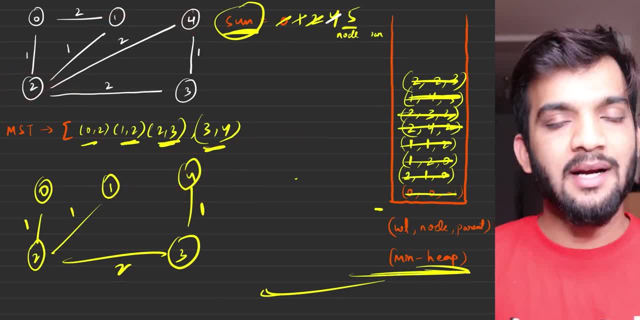 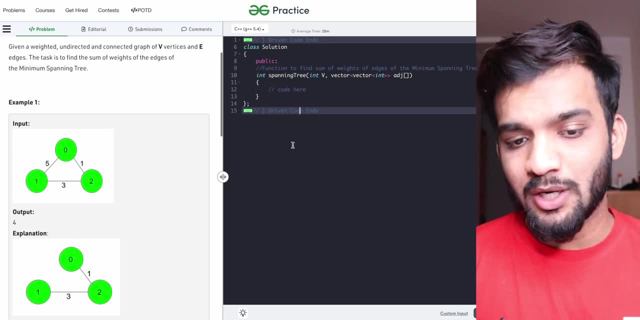 nodes, put them into the practical, keep on going, keep on going and ultimately you will get your mst. so i hope you've understood the entire explanation. now it's time to code it up. so, as usual, i'll be coding the c plus plus on the right, and you can find the exact, similar java solution on the left. 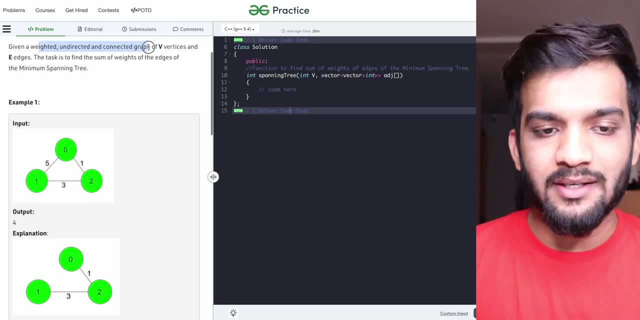 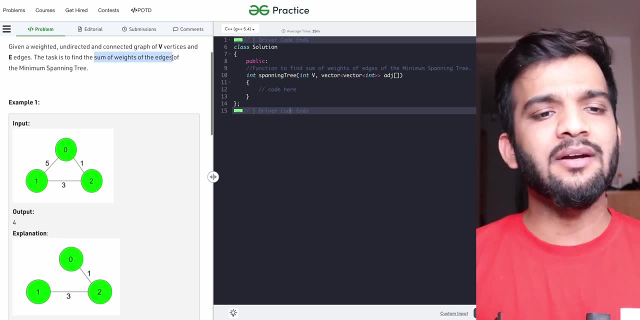 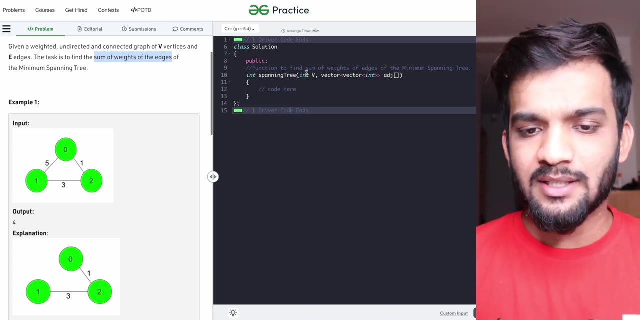 so what does the question state? uh, given an weighted, undirected, connected graph of v vertices and e edges, task is to find the sum of weights of the edges. they don't want you to find the minimum spanning tree, they want just the sum of the weights of the edges. so what i'll do is: i i've been given the v and uh the graph. 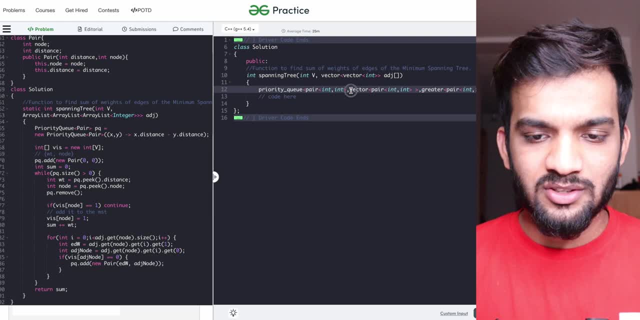 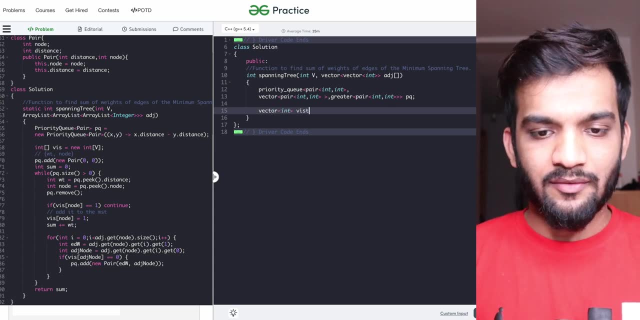 so i'll declare a priority queue at the first, because that is what i require. so this is how the priority queue will be, or the minimum heap. and what else do we require? we require a visited guy. so let's take a visited guy, if you remember, and i'll mark everything as zero and in the priority. 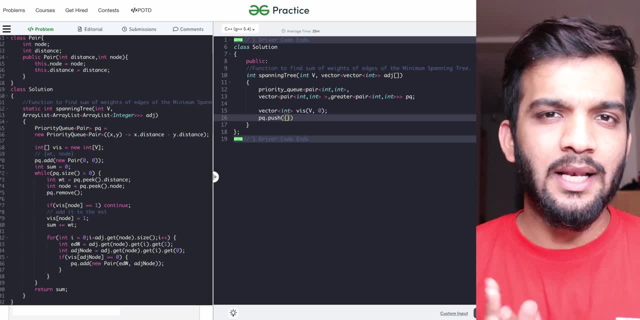 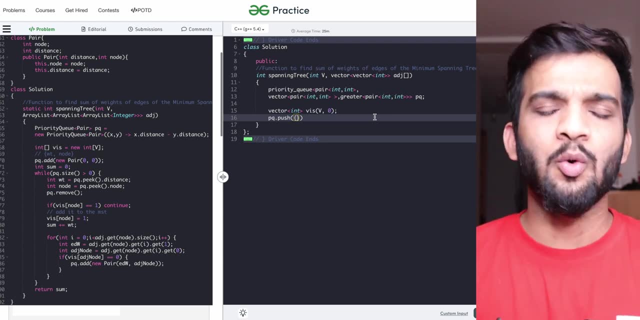 queue initially now over here. one thing i like to clarify. we just need the sum of weights of the goddess and with that, f of the m is equal to the sum of the minutes. so when you are asked for the sum of weights of the goddess and you are asked back to the m, s, t plus u of the m and your mc. 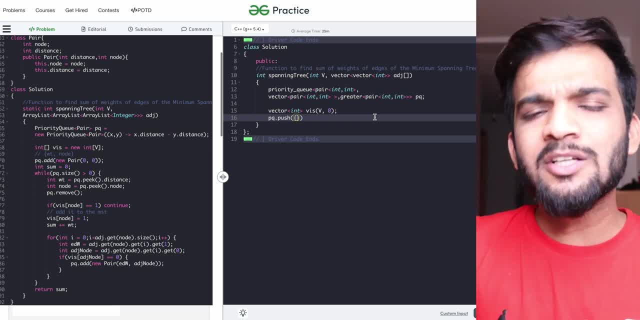 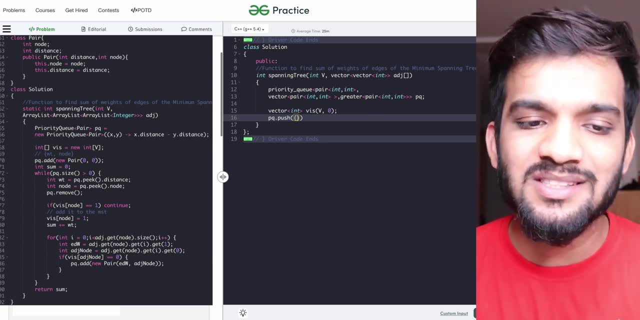 is equal to the m t minus n. so first we need to stake out the m s t that is equal to the sum of weights made by you. and now i know that you want to calculate this by taking the sum of weight of the roger dotento Delta, and I just have to take in the m s t dotnumber undieg that i just 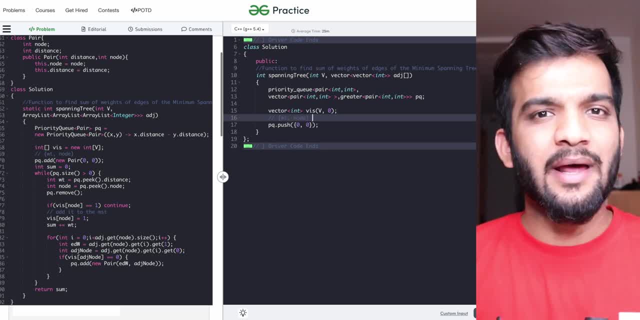 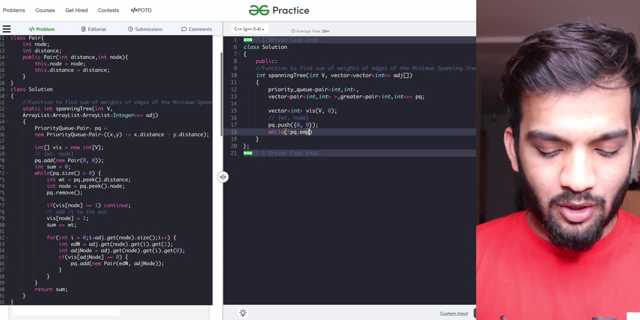 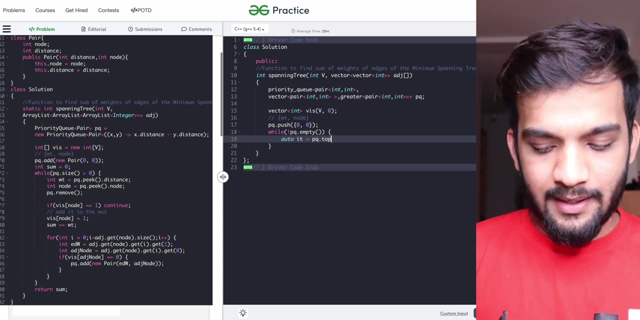 put everything, but i am taking 0. i have to take in the root division as well, so very easy. okay, you can go ahead and store the parent, okay, but over here we don't need anything. so what i'll be like, okay, while pqmt, that's the case. so what i'll get is auto of it is pqtop, okay, and at the same. 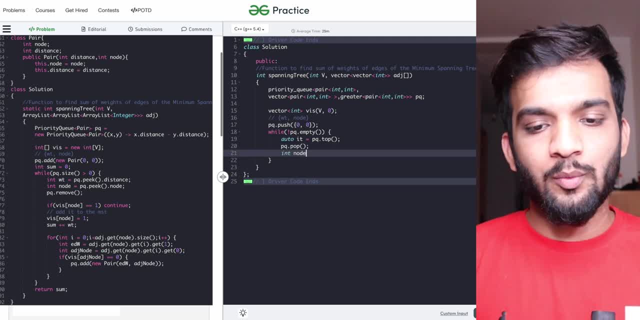 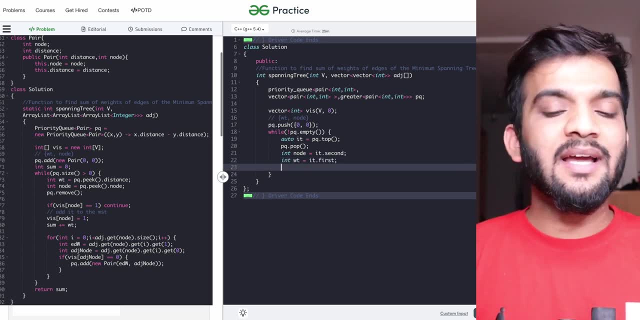 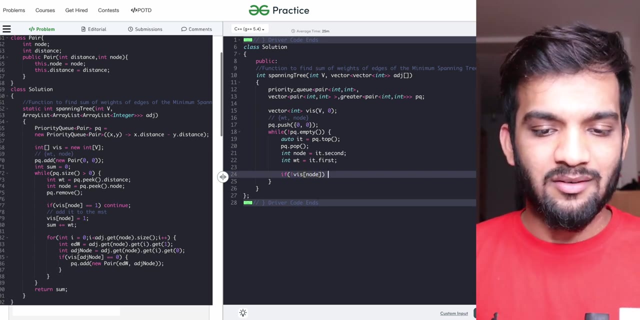 time i can do pqpop. now i can say the node will be at the second position. i'll get the node and i know one thing: the weight will be at the first position. now, something i know for sure is: if this node is already visited, that means it's already a part of the mst. so i'll say, hey, no need to do. 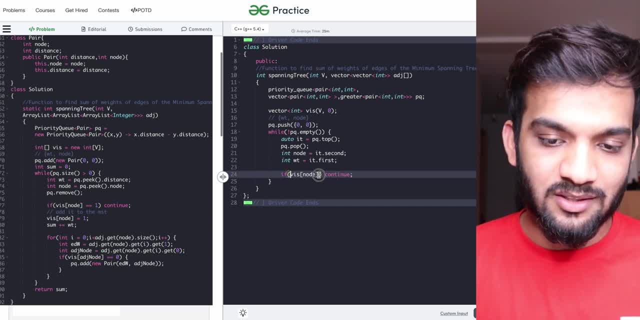 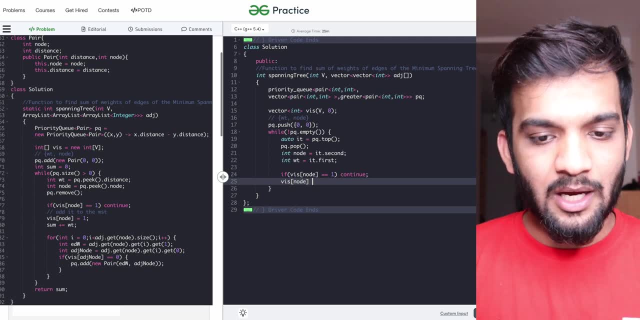 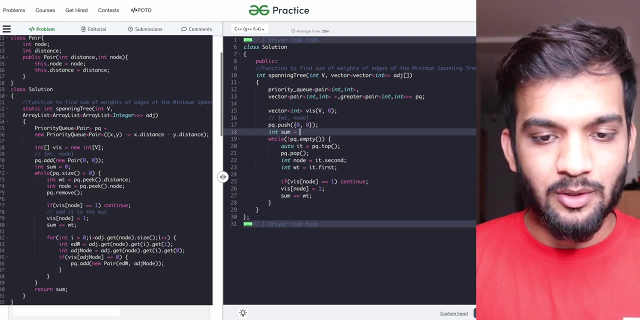 anything if it's already the part of the mst. or i can say, let's rather this: if it's already visited, let's go ahead, let's go out and get the next node. if it's not visited, i'll say, okay, come ahead, be a part of the mst, come ahead and give it to the sum. so probably i can declare something like sum equal. 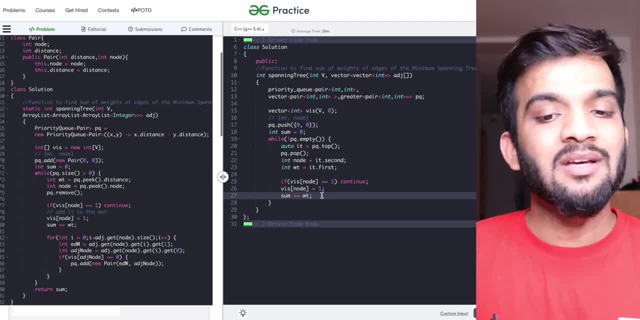 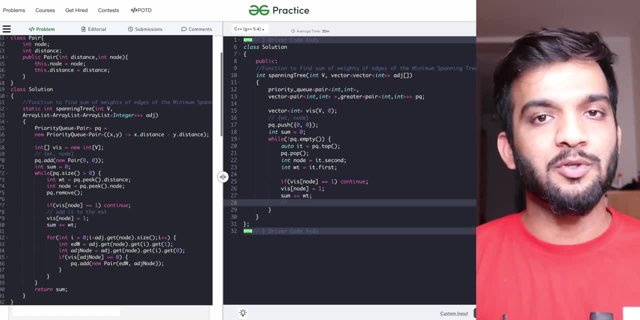 to zero. that's what i'll do. it'll be a part of the mst. in case someone would have asked you to get the mst, you can do that. you would have taken the parent and stored it in some list in this position. okay, but we don't need. 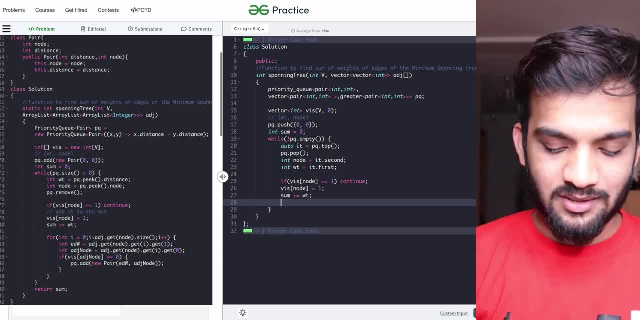 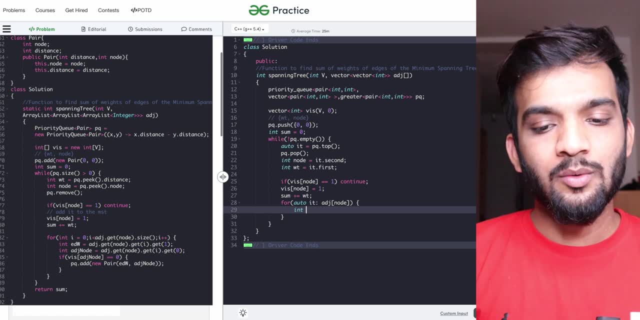 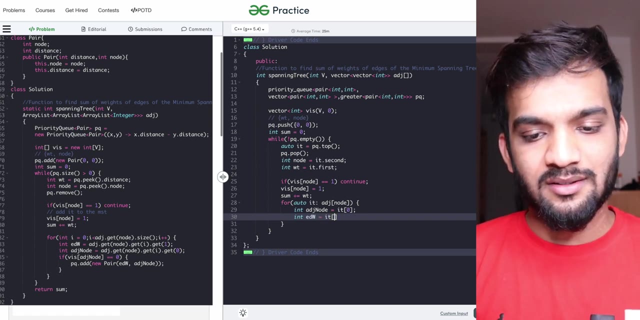 it now. what's the next thing? we've got the node: get all the adjacent guys- yes. how you get all the adjacent guys, very simple. i trade on all the adjacent guys, like this, and then where is the node? this guy, yes. and what's the edge weight of that guy? this one, right now. what do you need if? 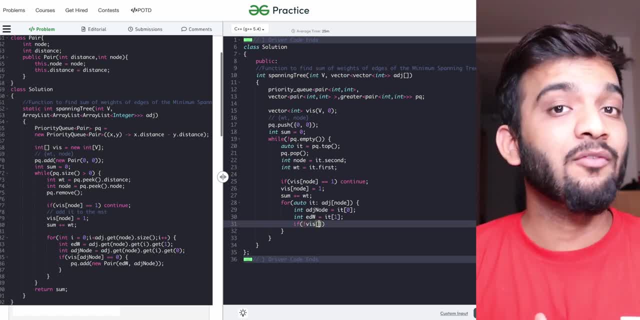 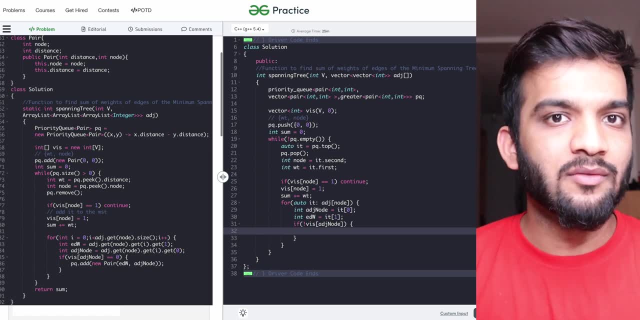 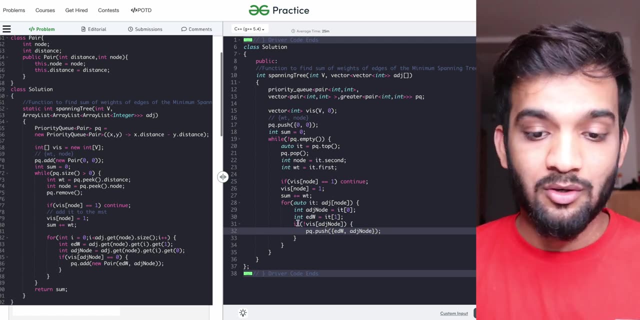 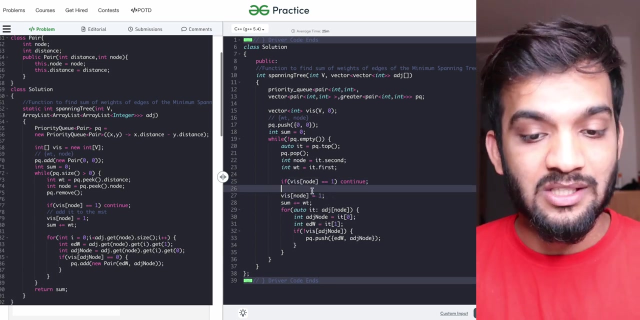 it's not visited or not a part of mst yet. if it's not a part of the mst yet, then i go ahead and say, okay, you're not a part of the mst. can you go ahead and get into the priority queue? simple, no need to market as visited. we market as visited only at this junction, when we add it to the mst. 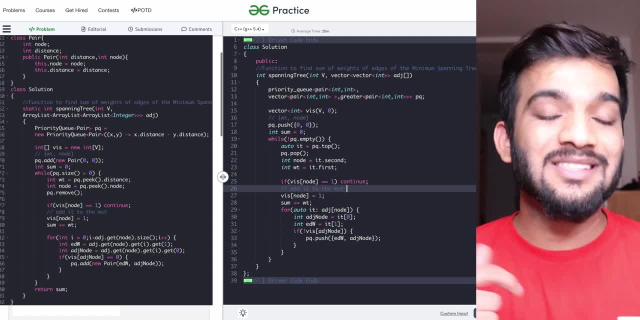 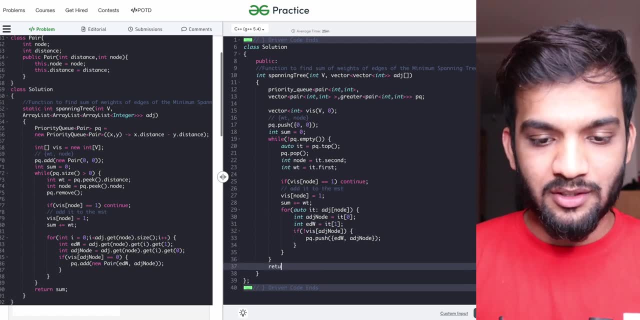 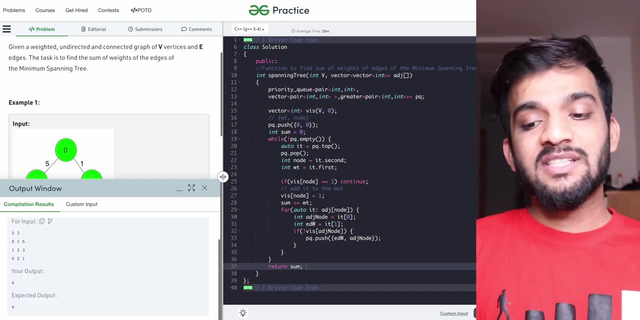 this is when i add it to the mst, that's when i you only do it, okay. so very simple. and once you've done this, you need to return the sum. so go ahead and return the sum. so i'll just go ahead and return the sum. so we see it's compiling fine. 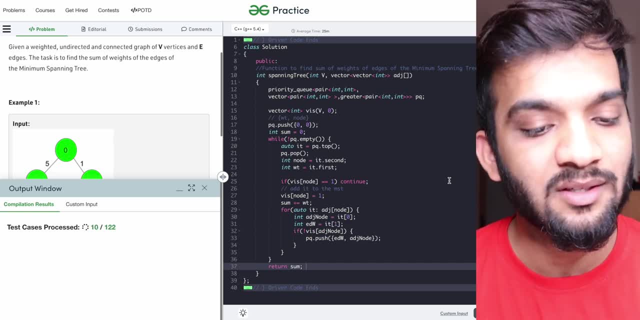 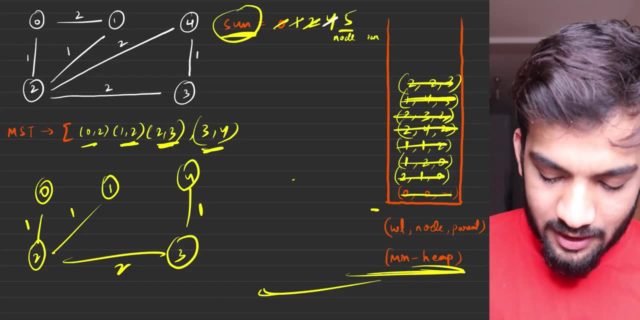 let's quickly submit this and see if it is running. all the test cases. we see, all the test cases are running fine. so the prims algorithm was very simple. i've written the code. i might be thinking, but striver, what is the intuition? the intuition is very simple, guys. you started with zero. 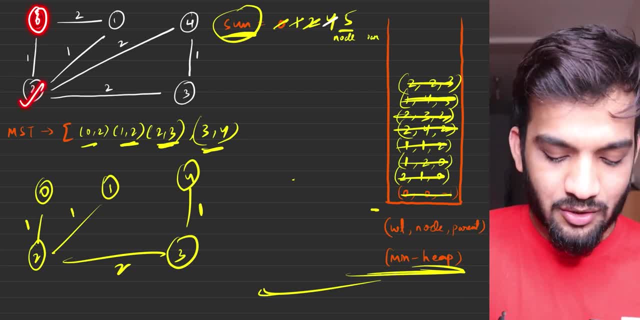 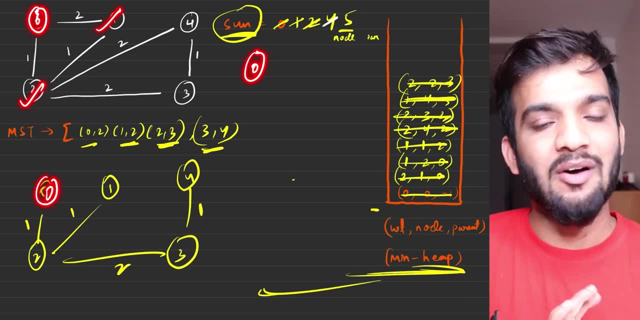 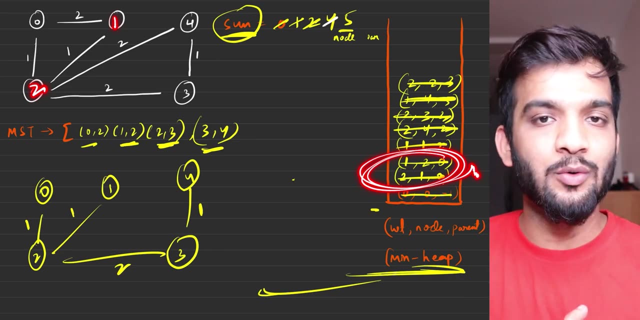 yes, and after that what did you do? you took the adjacent nodes right. so you basically start with the node and you know zero will be in mst, zero will be connected to someone for sure. so you just entered one and two into the priority queue, right and out of those, out of those, both adjacent in the 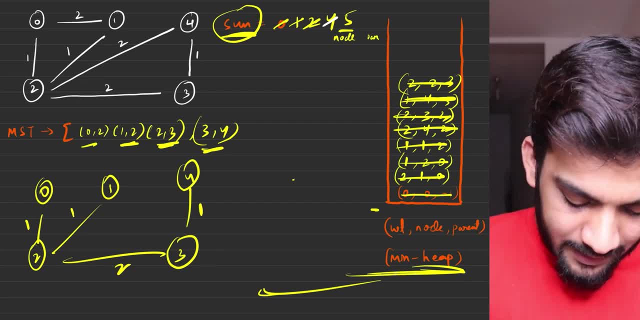 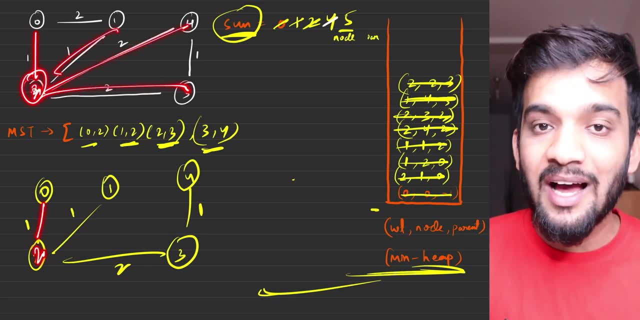 next step, you took the minimum, so it's a greedy. you took the minimum. that's why you got two and that's why this was added right. and next for two, you added all the adjacent nodes and you took the minimum again. for the next, you got the next minimum, which is this. so you added in this way: 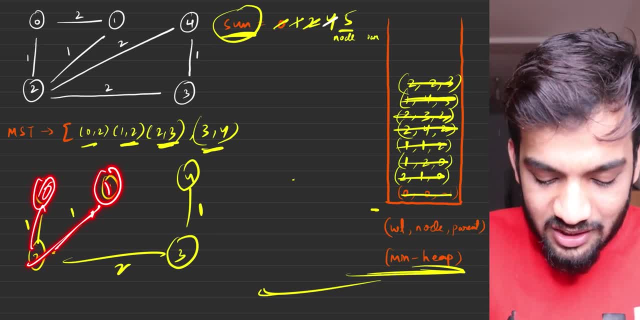 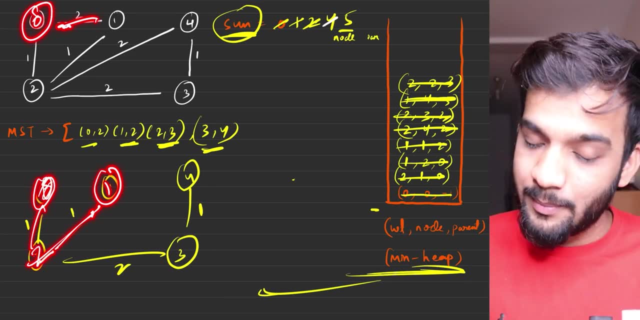 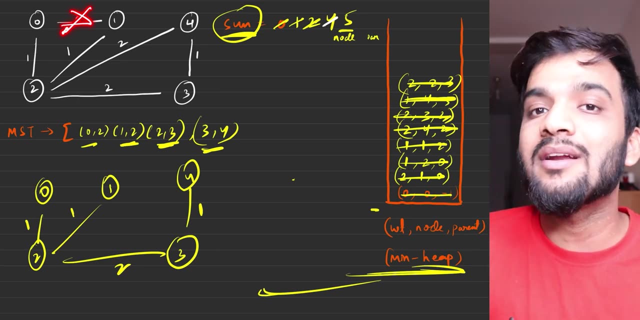 this one, but in the next, when you got this as minimum, it did not take it into account why. because zero was already in your mst, two was already in your mst, one was already in your mst, so there is no point of taking this. that's why this edge was ignored in your dryad. so the algorithm 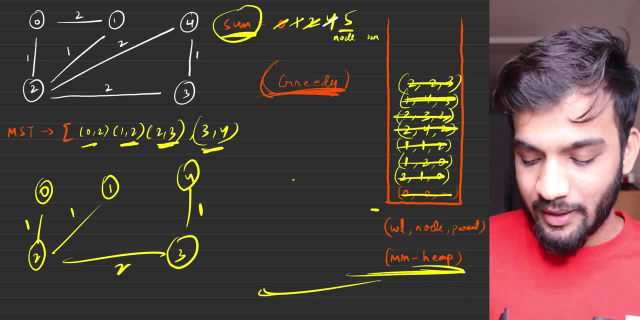 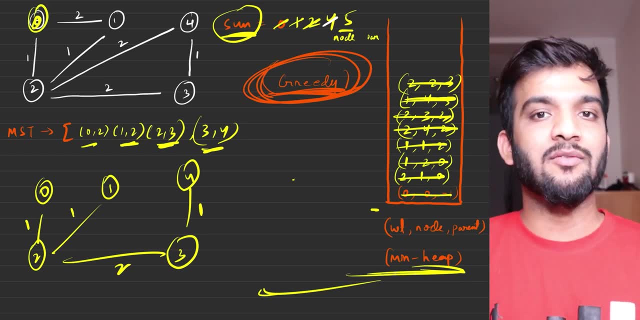 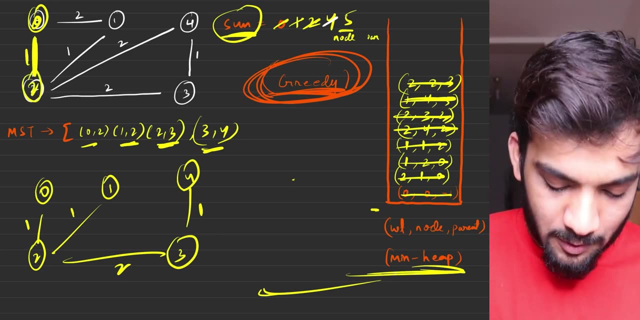 is very simple. so if someone does ask you about the intuition, you can tell him that greedy is the only way to get rid of it. so the algorithm will tell you how. we simply start with zero, because we know this will be the part of the mst and we we know one edge will be connected with zero, so get. 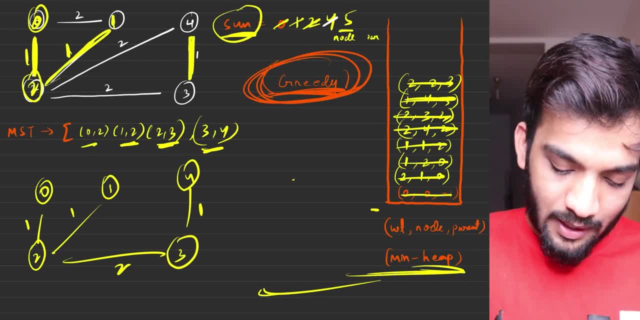 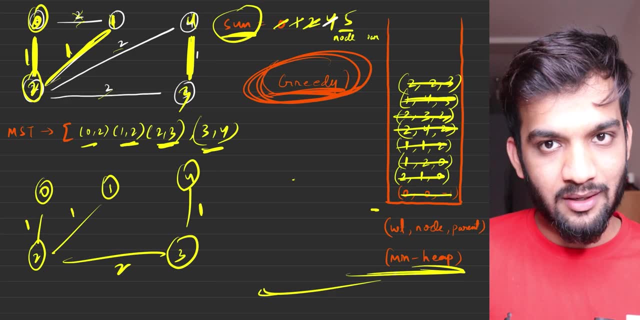 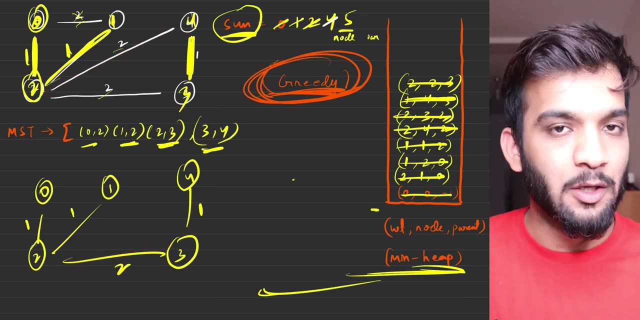 the minimal guy connected. next, get the next minimal guy connected. next minimal is one connected. next minimal is two, two, two. but this will not be connected because zero one is connected right. so the next guy: either you can take this two or this two. anyone you can take this or you can take. 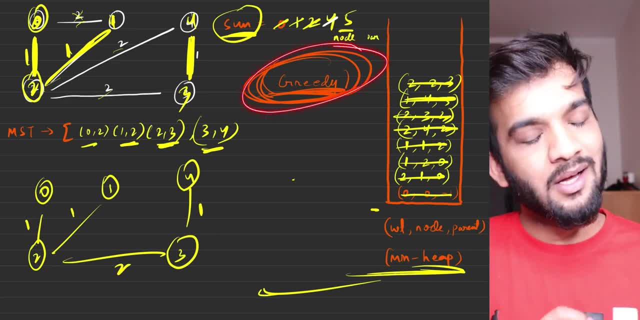 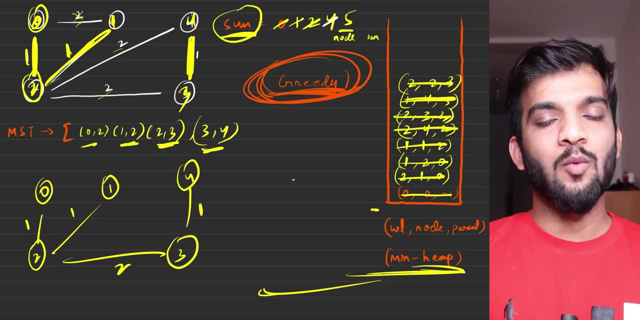 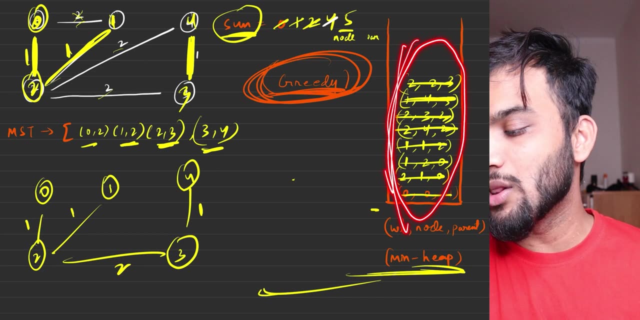 work fine. so this is what the intuition is: greedy. i just followed a simple greedy algorithm and that is the intuition behind solving this problem now. now you must be thinking: what is the time? complexity of this particular algorithm. so, if you carefully observe, we're actually running for all. 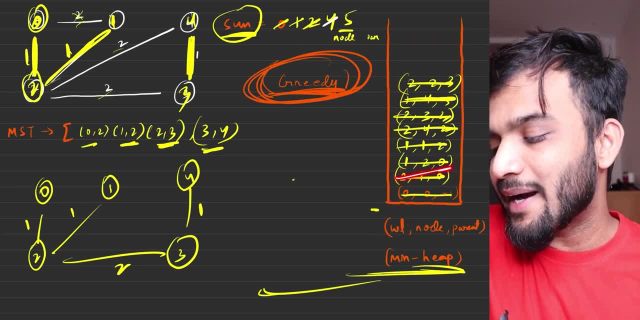 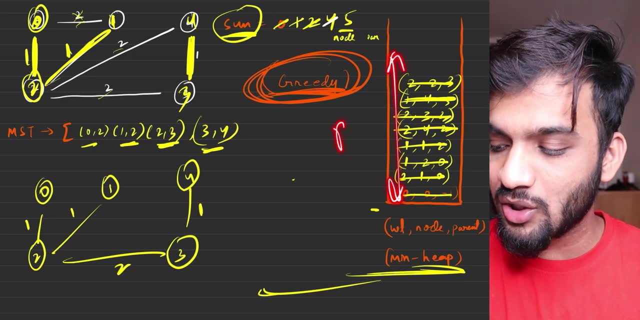 the edges in the priority queue. so the number of iterations in the priority queue will be the number of edges or somewhere near about that at the worst case. so i can say the iteration is definitely bigger of e. so i can say this: while loop will definitely run for e times and there is a priority. 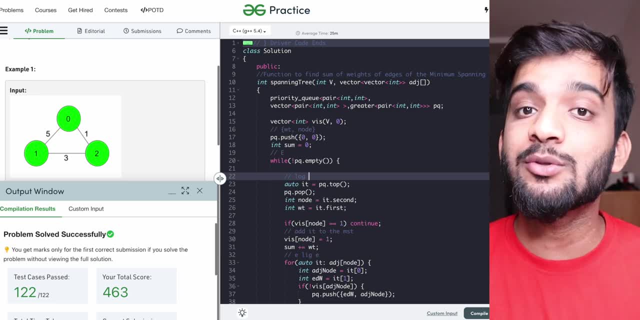 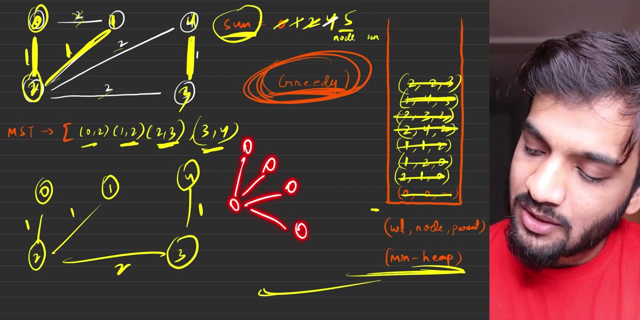 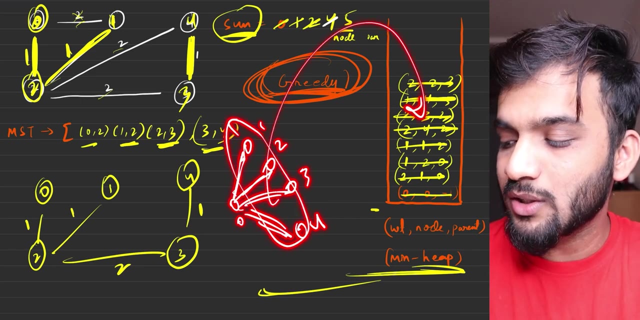 queue top, which will take logarithmic of priority queue size. what can be the worst case size? imagine a graph like this. imagine a graph like this: and this is zero, and this is one, this is two, three, four. so the first time it can have all the edges in the priority queue at the worst case, right. so